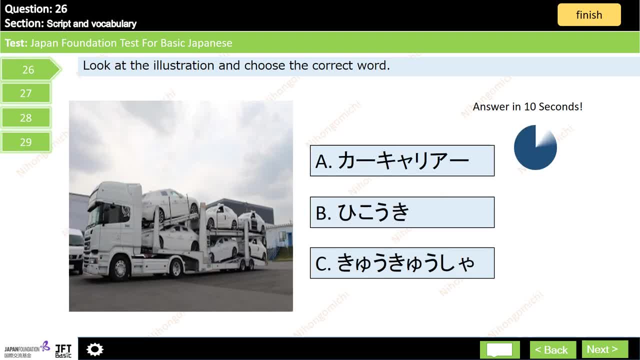 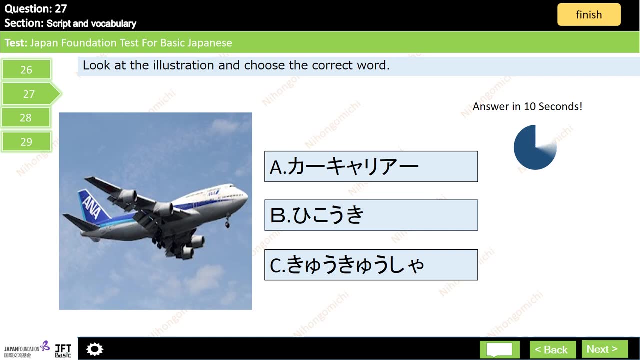 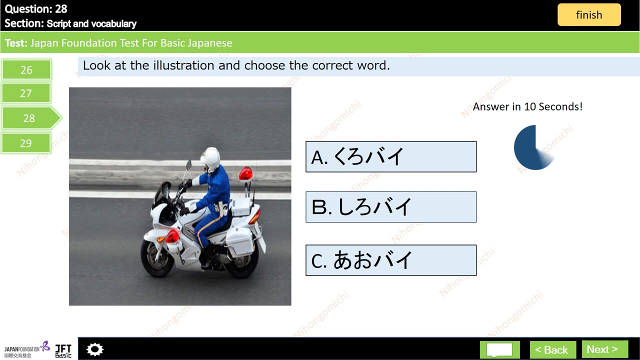 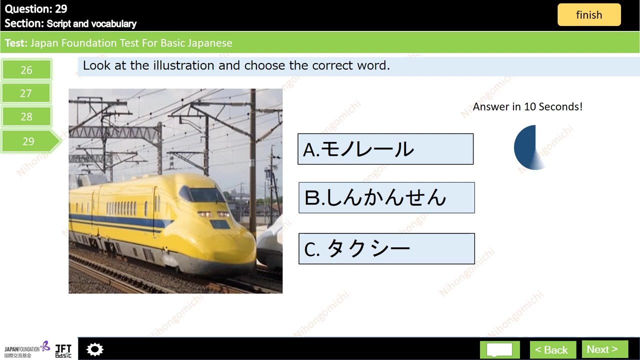 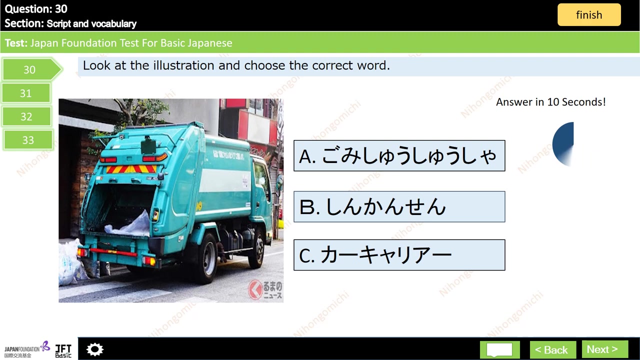 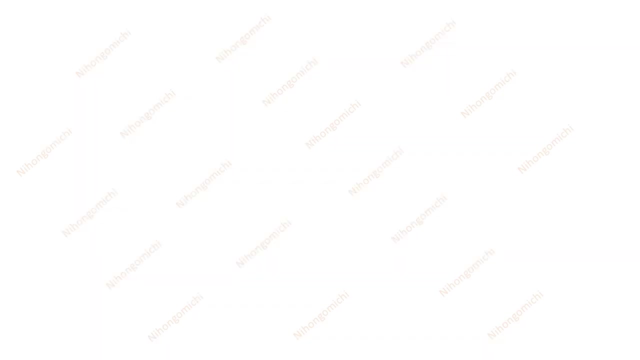 Thank you for watching. Thank you for watching. Thank you for watching.